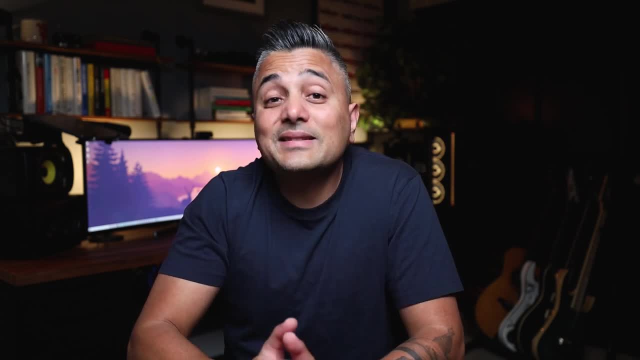 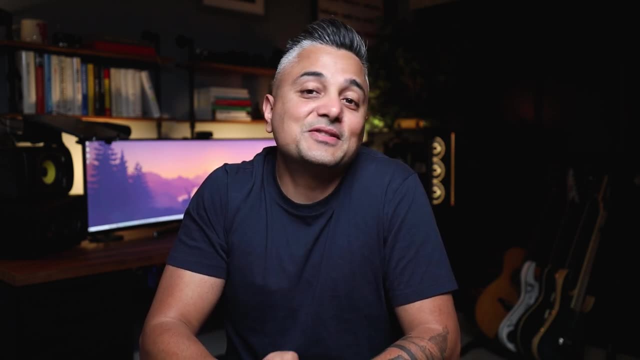 is also frustrating. So before you begin work, break down your tasks into a bunch of smaller subtasks. Let's pick a simple example and use it throughout the video so you can get a good sense of how you can manage your project. Let's say your task is to create an internal polling system for 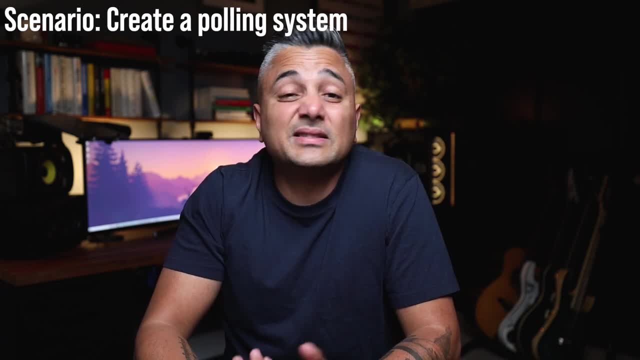 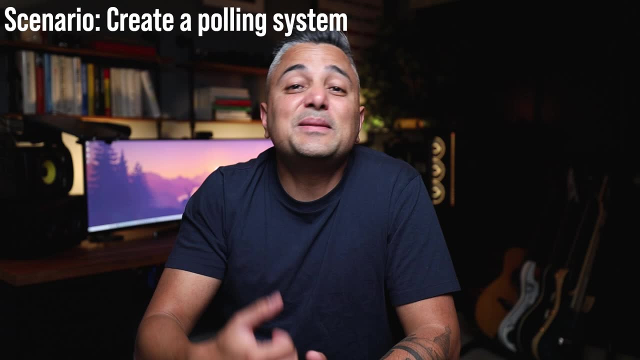 your team. This polling system will be used by your team to decide on various things like voting for a framework to use on a project, voting on a place to eat for a morale event- Basically, any time there are some multiple options and your team needs to vote on their choices. 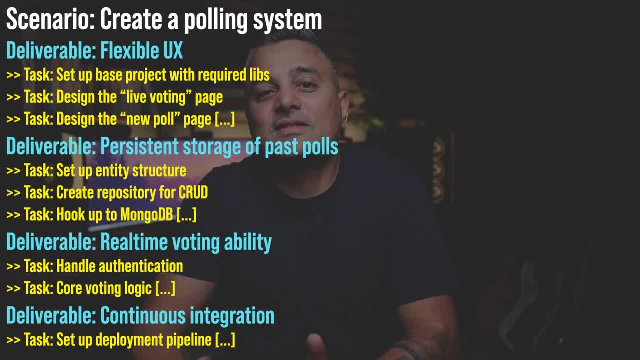 Okay, so you have a high-level task, but you can't just say, okay, I'm going to start building this. Spend some time thinking about the subparts of this project. A good rule of thumb is to decompose your high-level tasks into subtasks that each take roughly three days or less to finish. 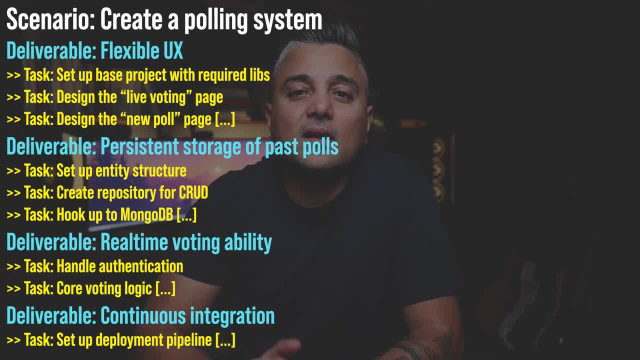 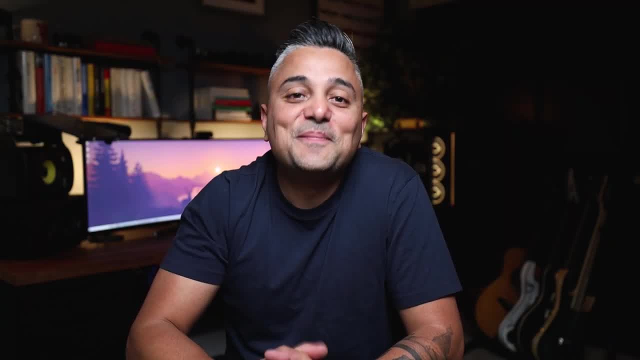 If a task takes longer than that, it needs to be broken down into further subtasks. But how do you decide how long something takes before actually even doing it? Well, that's the next step: Estimation As you decompose your task. 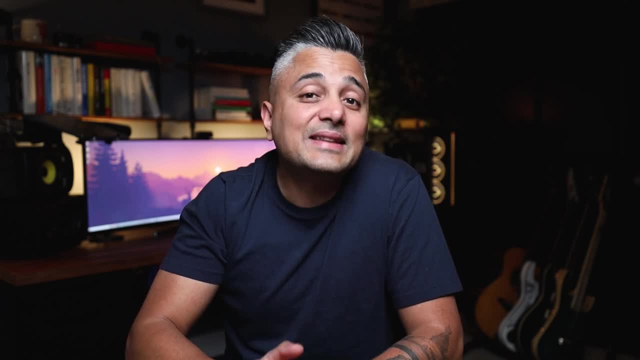 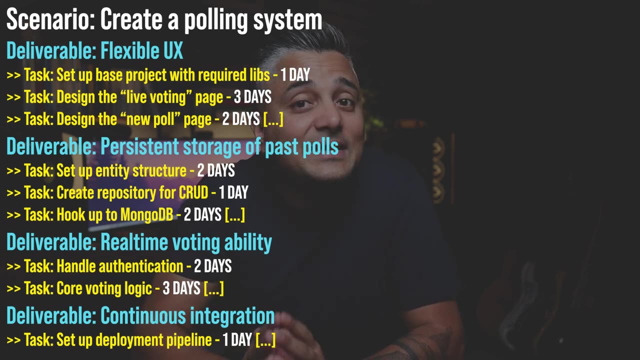 you will need to make an educated estimation on how long it will likely take you to complete. If it's a project that is new to you, your estimations may be inaccurate, and that's okay. Even if you're wildly guessing, you should still estimate, Because when you finish a task, you'll also record how long it takes you to complete it. Your strategy is to estimate how long it takes for your tasks to complete. If your project is new to you, your estimations may be inaccurate, And that's okay. Even if you are wildly guessing, you should still estimate. 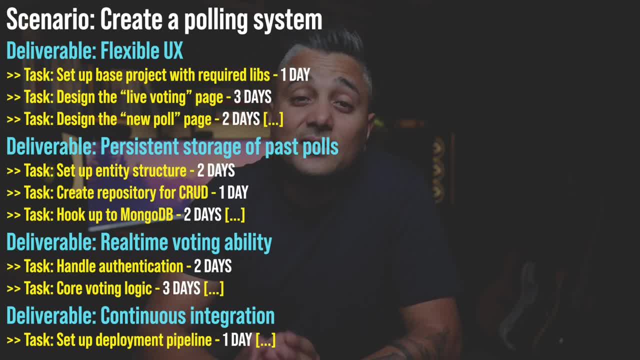 Because when you finish a task, you'll also record how long it will take you to complete it. long it actually took you to complete the task At that moment. three things can happen. You estimated correctly, you thought it would take you way longer than it actually took you, or it took. 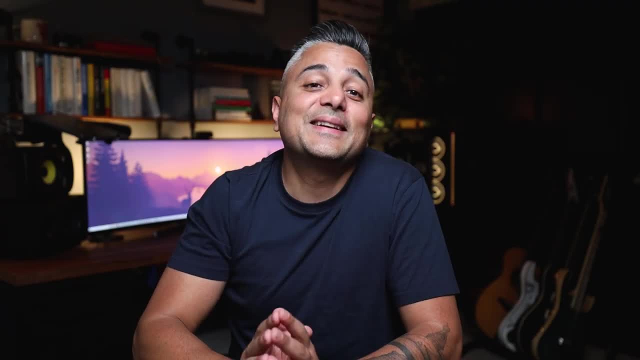 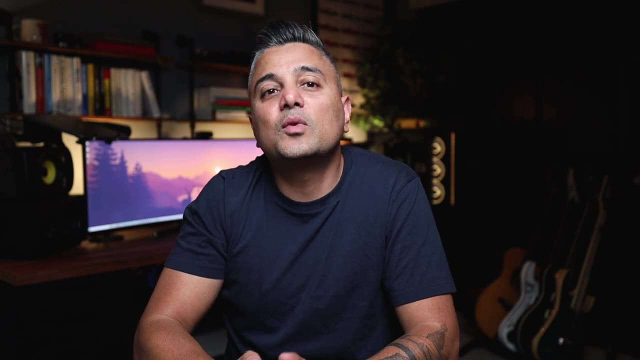 you way longer than you actually thought. If you estimated correctly, great job. If you're off at the end of the sprint, you should spend time reflecting on why you were off. The goal here is to learn what you can do to improve your estimations and avoid doing things that throw. 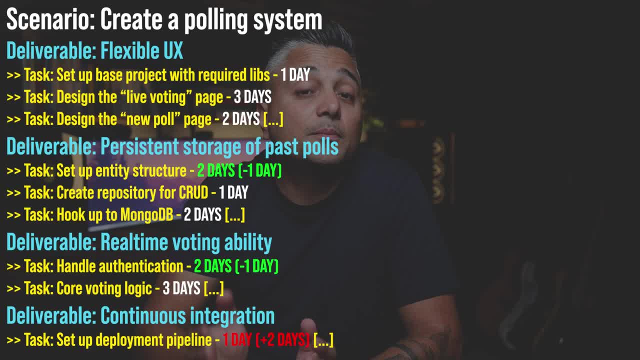 you off. For example, let's say that one of your tasks for your polling system was to create a continuous integration pipeline so that any code changes in the future can automatically go through the build, test and deployment processes, And you thought it would be relatively simple and take you. 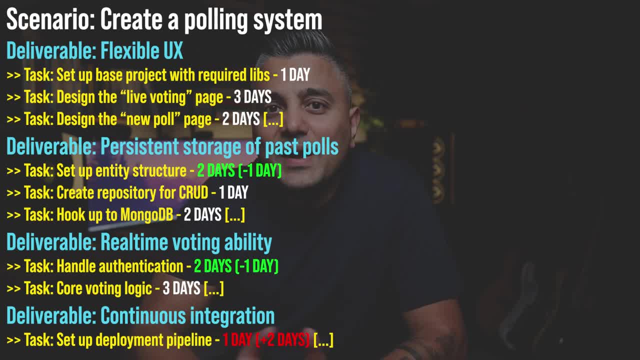 a day to implement. However, it takes you three days. Figure out why. Why did you think that it was easy? Maybe you got stuck on something for one entire day. Maybe next time you should ask the moment you are stuck for one, two hours for help from someone else. Maybe you thought the pipeline. 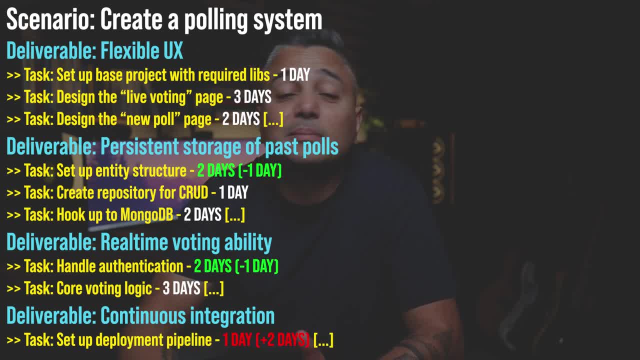 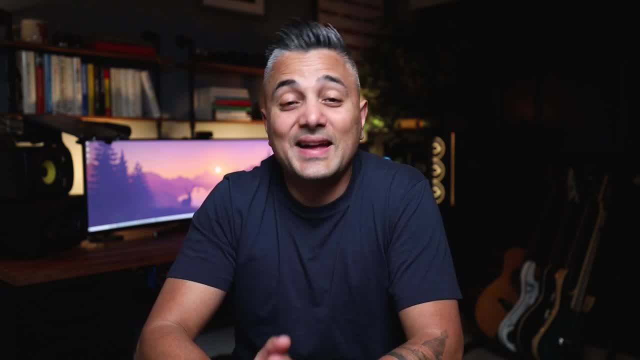 was based on JSON and it used YAML instead, and you had to pick up the new format. These are all great learnings, And the more you do this estimation reflection process, the better your anticipation becomes And, as a result, your estimations get very accurate. Task decomposition lets you figure out. 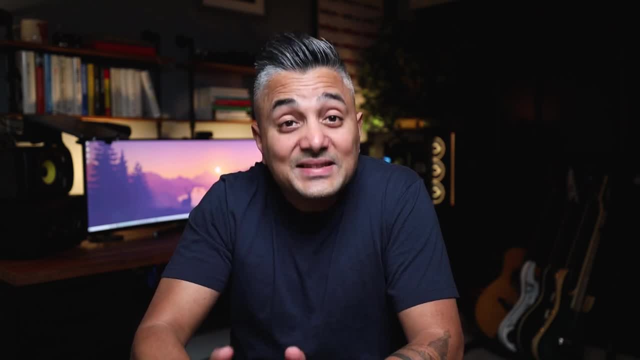 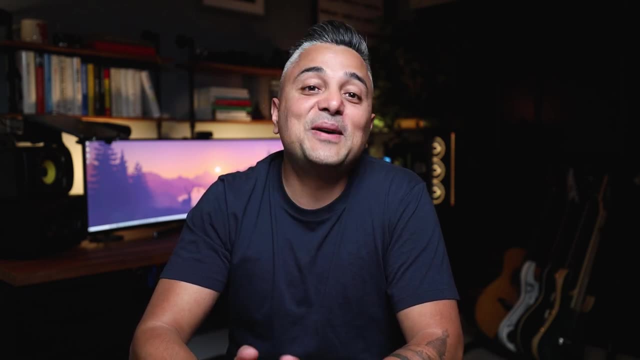 what exactly you need to do. at a very granular level, Estimation lets you know exactly how long these tasks will take you to complete. In an ideal world, the amount of time you have and the amount of work you have to do are exactly the same. However, in a real world, you will always have. 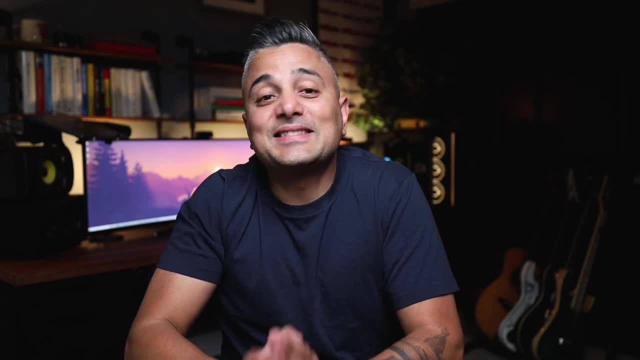 more work compared to the amount of time you have. So, even though you have your task decomposed and estimated, you still have a lot of work to do, And that's exactly what you need to do, And that's exactly what you need to do. So, even though you have your task decomposed and estimated, you will 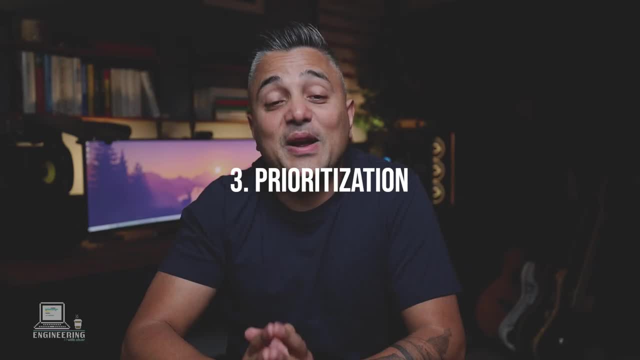 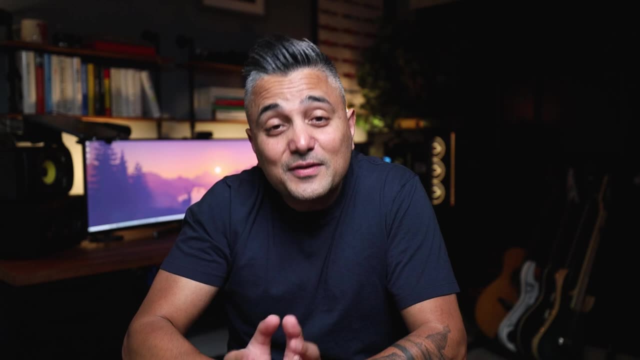 still need to prioritize them, Which takes me to step number three, prioritization. When we think about priority, we generally think of severity, as in low, medium, high. That works for general bucketing, but in terms of proper task and time management. 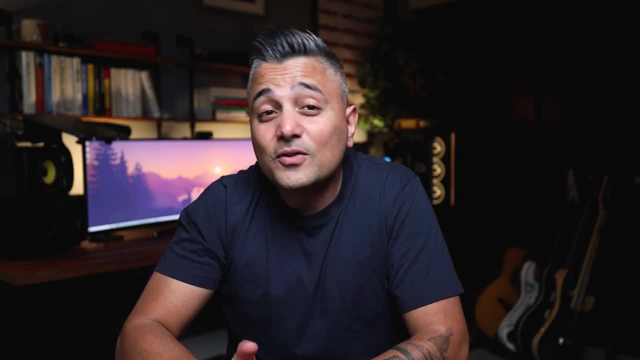 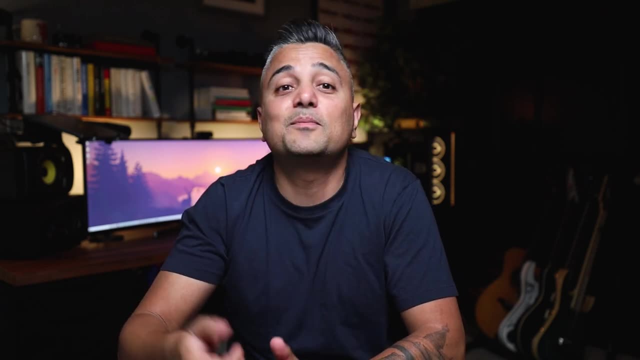 every single one of your tasks should have a rank. Rank not only helps you prioritize your work, but also quickly visualize the dependency. For example, the task to create a deployment pipeline for your polling system cannot be rank one because you will need to essentially finish. 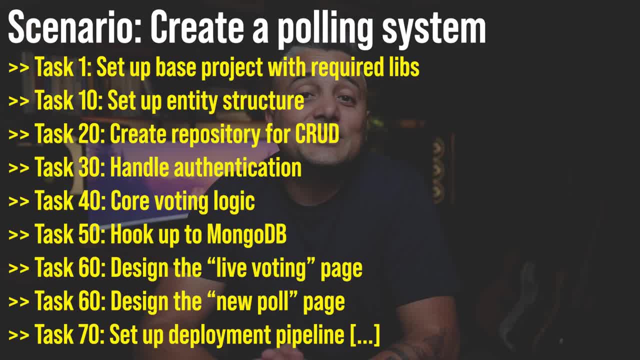 enough tasks to give you at least one or two hours to complete the task, So you need to some code to deploy. A good idea is to start by ranking every task in intervals of 10.. For example, the first task you do should be rank one. the second task should be rank 10,. 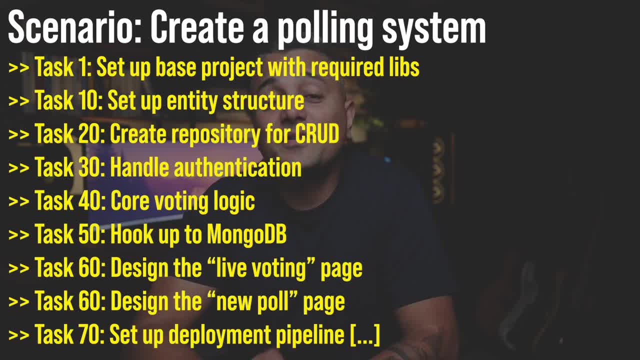 third should be rank 30, so on and so forth. That way you have enough space to insert tasks in between or move them around. There is no hard and fast rule here. The idea is to have an ordering that describes priority as well as the dependency of your work. 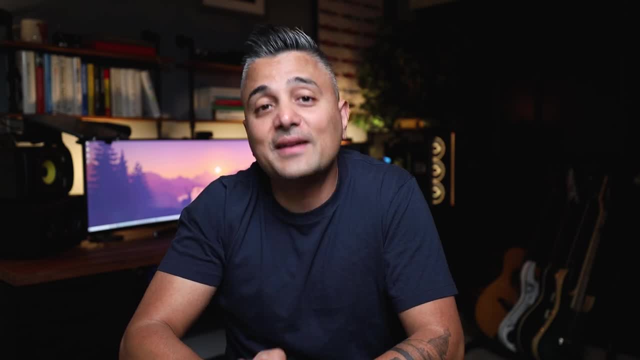 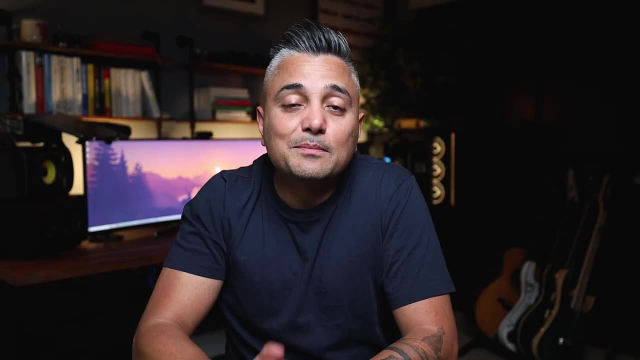 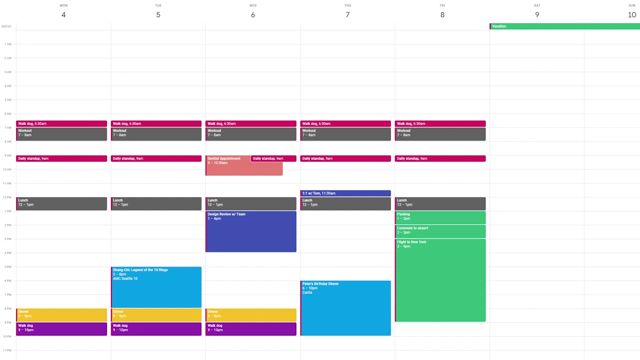 Okay, so you've decomposed your tasks, estimated them and prioritized them. The only thing left to do is to organize them, which is step number four. Organization is the simplest step. Open your calendar and block out the times where you won't be able to work on these tasks. Meetings: lunch. 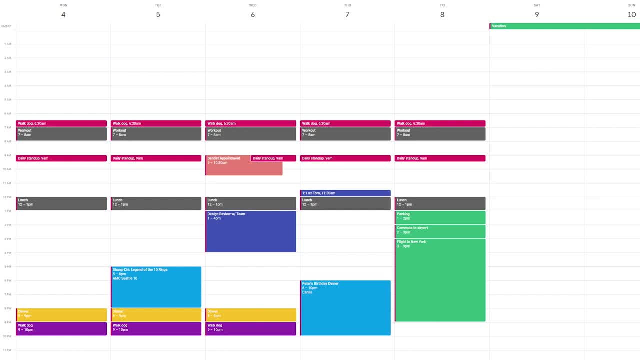 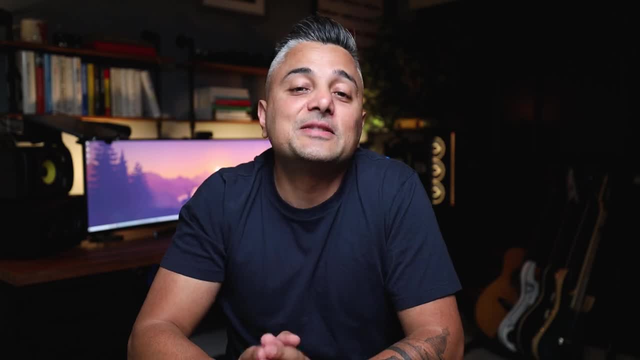 workout your personal and family time, vacation times where you simply want to disconnect, dentist appointments, whatever else there is. Now start at the beginning of your sprint and start filling in the empty spaces, beginning with your highest ranked tasks and moving down the list. 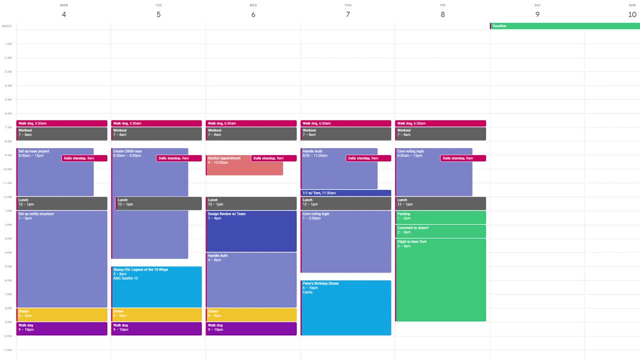 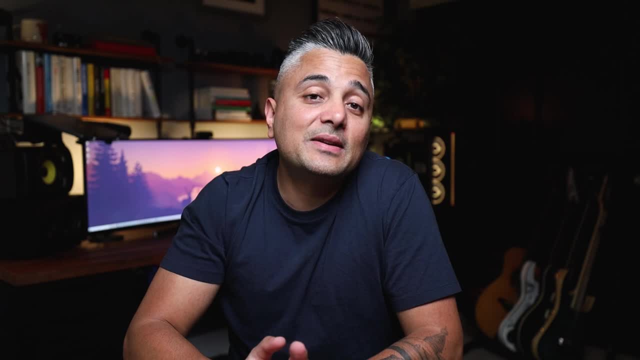 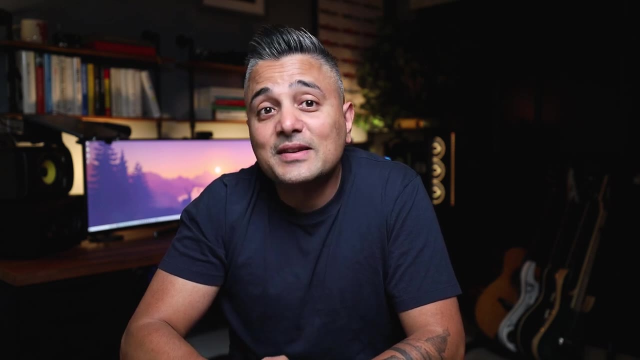 Every few tasks, leave some buffer of free time so that you have time to adapt and adjust should things not go according to plan, And that's it. The day before beginning a new sprint, spend 30 minutes doing your decomposition, estimation, prioritization and organization. Once you've done that, for the rest of the sprint. 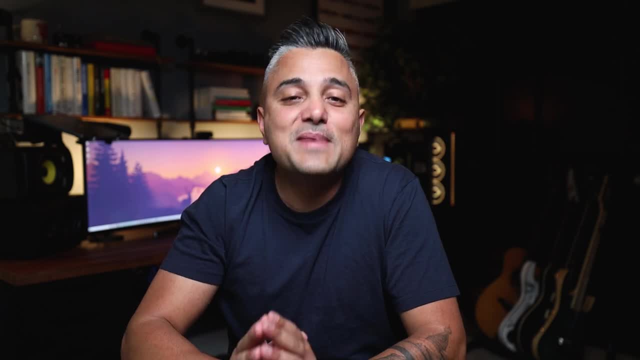 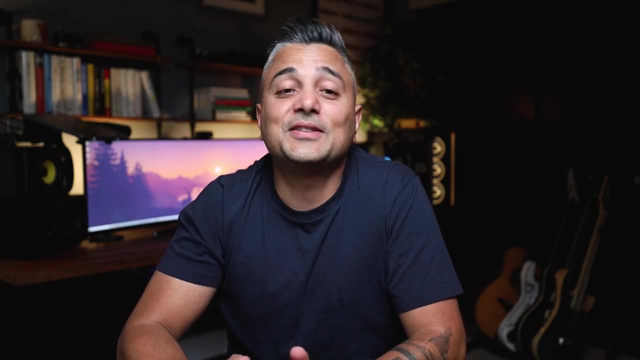 all you need to do is just follow the calendar, and you don't have to spend a minute thinking about managing time, because you've put in the effort in the beginning to do that. All you need to do is pick up a task that your calendar says on the times that your calendar says. 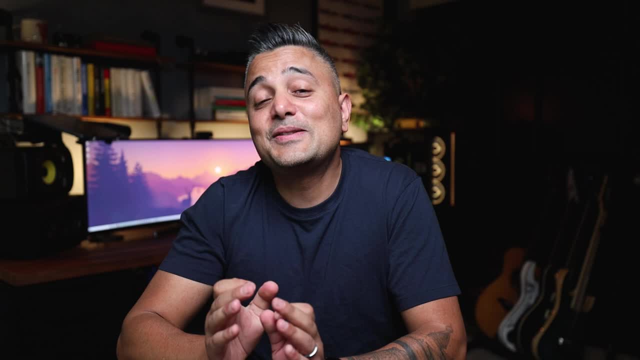 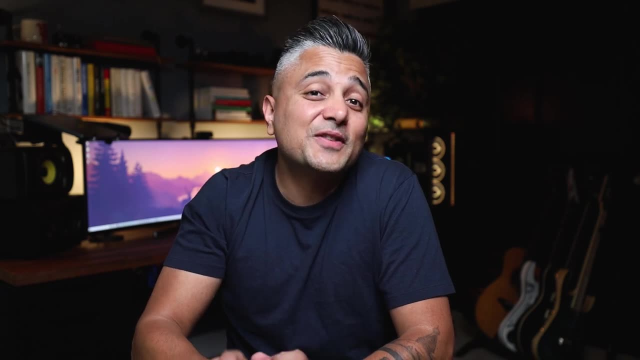 The key takeaway here is that the best way to manage your time is by not trying to manage your time all the time, But do remember to reflect on what you did at the end of your sprint so that you can figure out the things that worked and the things that did not work. You want to learn and continually improve. 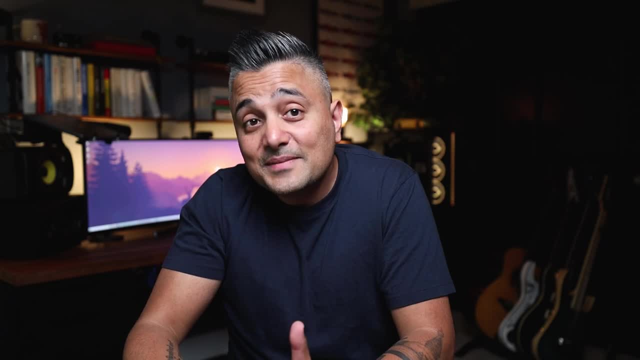 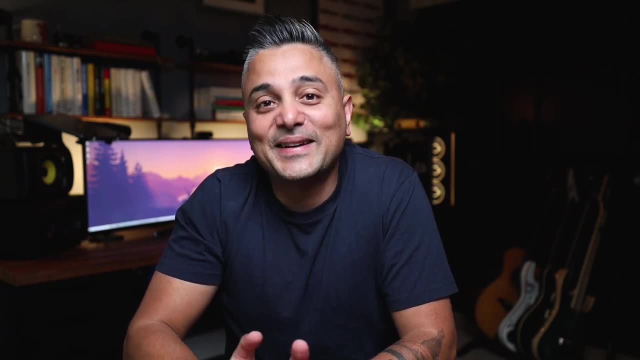 your process. That way, your decomposition gets better, your estimations get better, your prioritization gets better and your organization gets better. And guess what happens when all four things align perfectly? You get the most out of your time, And that's what time management is. 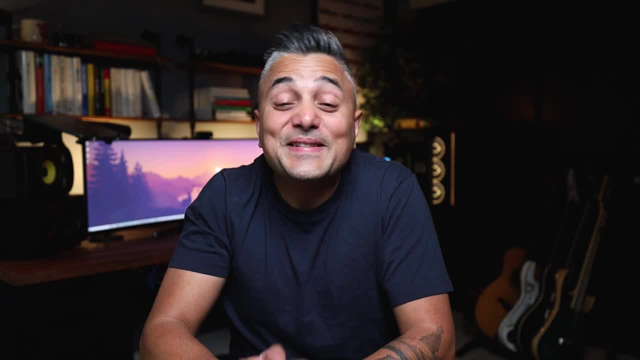 Obviously, this is a very simplified version of a sprint, one that has very little overhead and very easy to do, especially if you're starting out. However, there are many other techniques you can follow to get even more out of your time, But it would kind of be ironic to spend weeks or months of time. 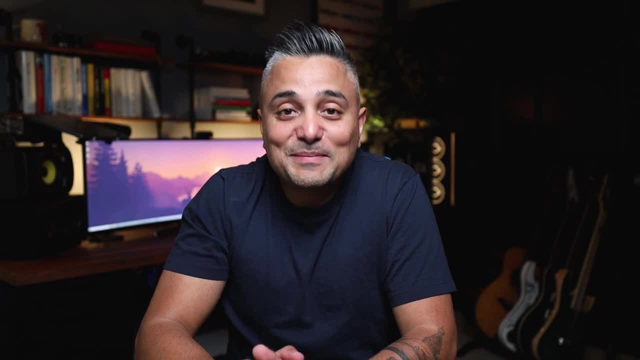 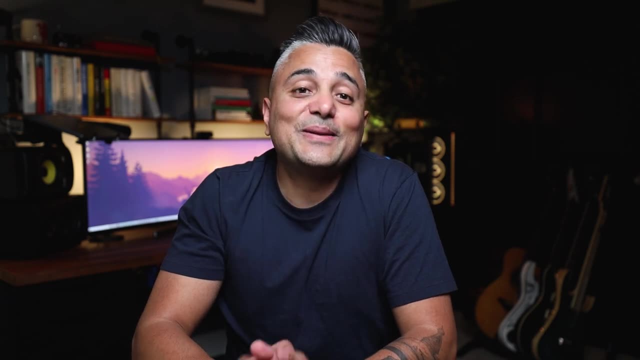 learning about time management. That is why Skillshare is a great place to learn about things like time management, because their classes are not only taught by amazing professionals, but they're also all about an hour in length. Skillshare is an online learning community for creative and curious people, where millions 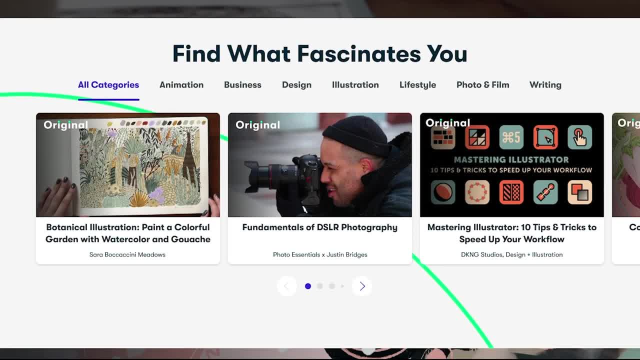 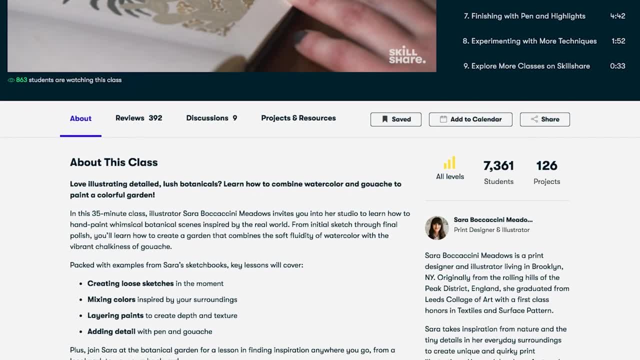 come together to take the next step in their creative journey. They offer thousands of inspiring classes for lifelong learners on a variety of topics, including web development, design, freelancing music, communication, to name a few. There are classes for every skill level, whether you're a beginner or a pro.